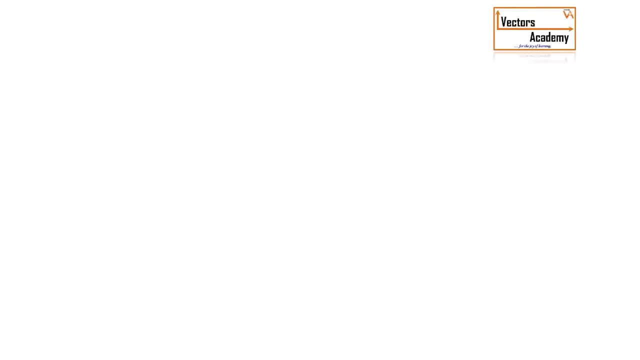 We will now study a new method to solve linear equations, That is, the graphical method. We have already studied how to draw a graph of a line. Now suppose there are two equations which are given. We will consider the first equation, that is, x plus y equal to 6.. Now 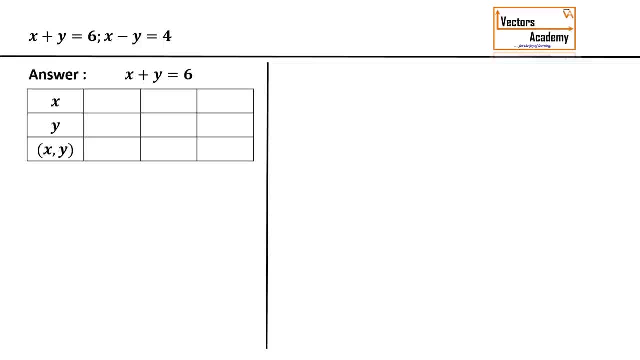 we have to prepare a table which contains the x coordinate, y coordinate and the point that is, the x and the y coordinate. We will assume three values of x, Suppose we assume it as 0,, 2 and 4.. We will substitute these values of x one by one in the given equation. 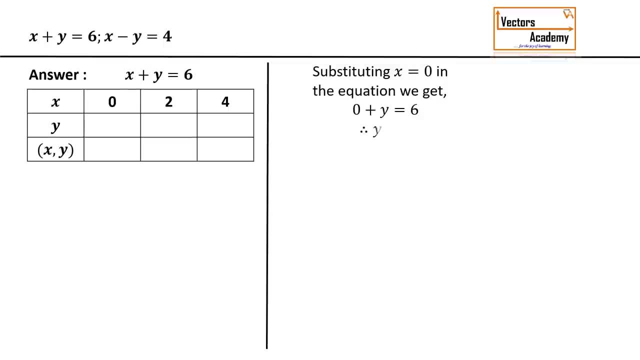 So if I substitute 0 in the given equation, I will get: 0 plus y is equal to 6 and y will be equal to 6.. I will write it down in the table, For x equal to 0, y is equal to 6.. 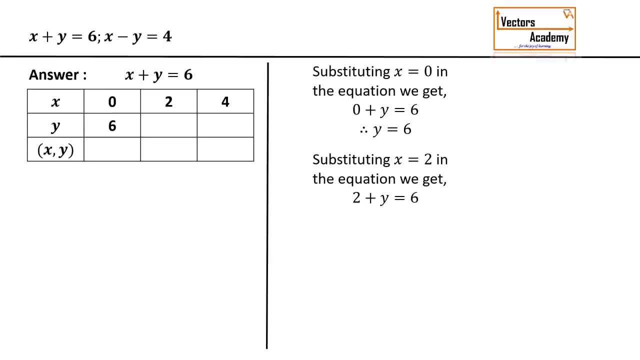 In the same way, I will take the second value of x, That is x equal to 0. I will write it down in the table. I will take the third value of x. I will substitute it in the given equation. What I will get is 2 plus y is equal to 6 and y will be equal to 4.. Again, I will write. 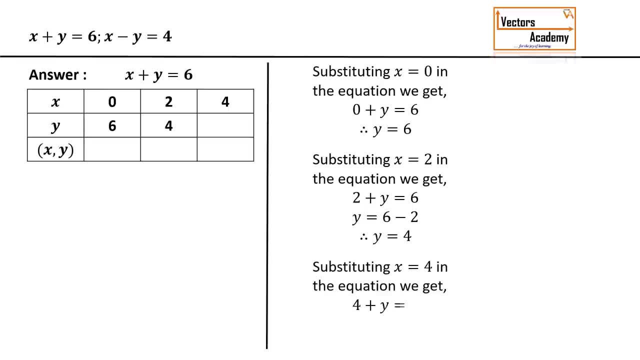 it down in the table. Exactly in the same way, I will take the third value of x substitute in the given equation and find out the value of y and write it down in the table. So once we have completed the table, we can now plot the point. The first point is 0, 6.. The second 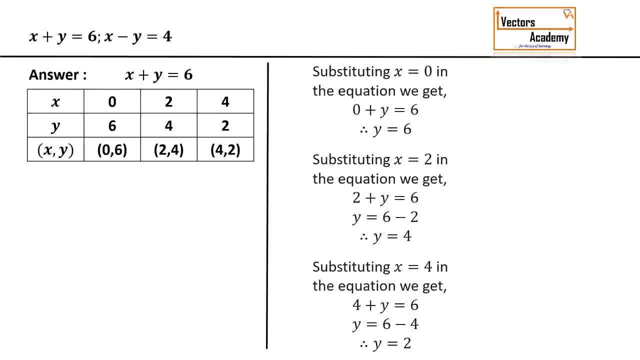 is 2, 4 and the third is 4, 2.. So, exactly in the same way, we have to make the table for the second line as well. Hence, we will assume any three values of x. Make sure, when you assume the values, you don't. 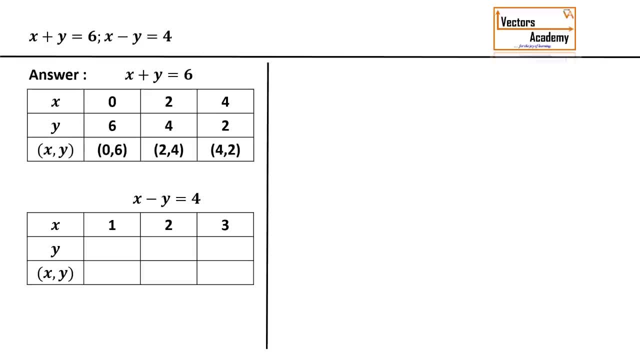 get a fractional answer, because that won't be easy to plot on the graph. Ok, so we will take x equal to 1 and substitute in the given equation, That is, 1 minus y is equal to 4.. Solving it, I will get the value of y as minus 3.. 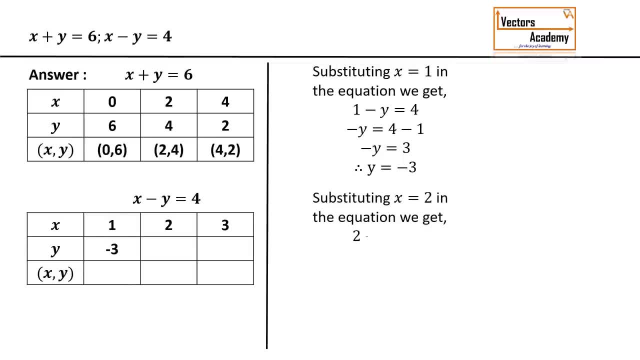 and write it down in the table. I'll take the second value of x, that is x equal to 2, and substitute in the equation Again, solve it. I'll get the value of y and exactly in the same way I'll substitute x equal to 3. that is the third value in. 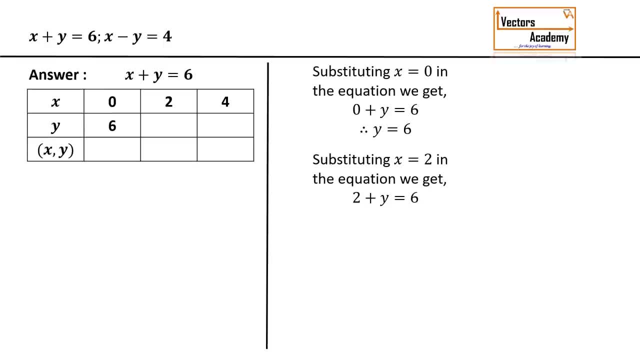 way, I will take second value of X, das is X equal to 0.. Now, for same value, X is equal, equal to 2, and substitute in the given equation. What I'll get is 2 plus y is equal to 6 and y. 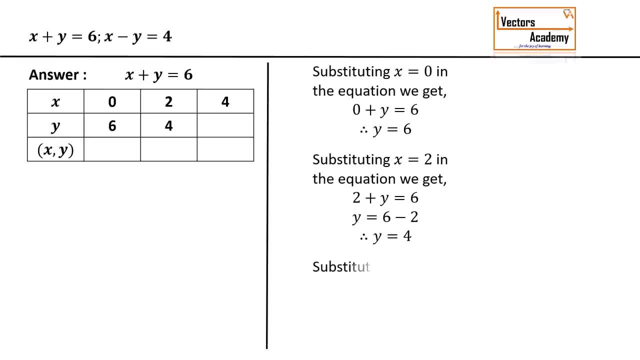 will be equal to 4.. Again, I'll write it down in the table. Exactly in the same way, I'll take the third value of x, substitute in the given equation and find out the value of y and write it down in the table. So once we have completed the table, we can now plot the point. The first point is 0,6,. 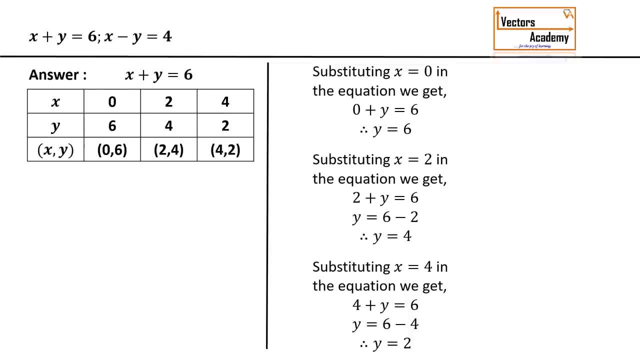 the second is 2,4 and the third is 4,2.. Exactly in the same way, we have to make the table for the second line as well. Hence we'll assume any three values of x. Make sure, when you assume the. 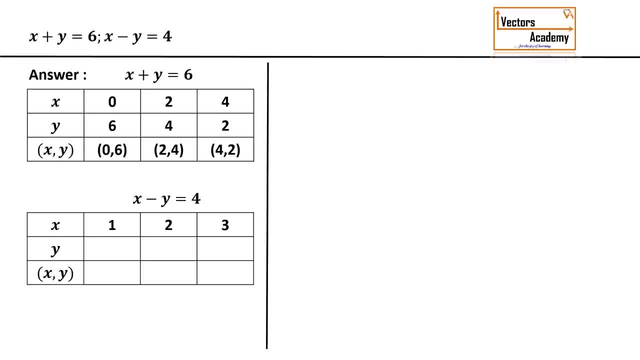 values. you don't get a fractional answer because that won't be easy to plot on the graph. Okay, so we'll take x equal to 1 and substitute in the given equation, that is, 1 minus y is equal to 4.. Solving it, I will get the value of y as minus 3 and write it down in the table. I'll take the 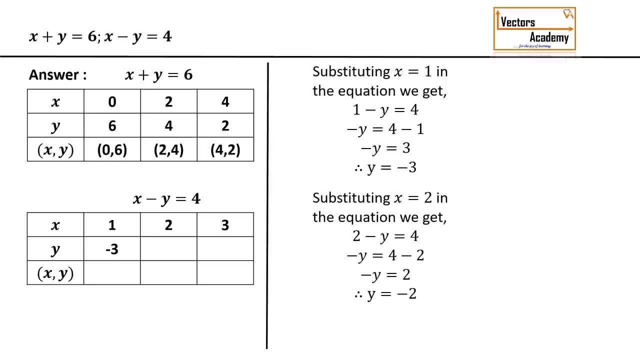 second value of x, that is x equal to 2, and substitute in the equation: Again, solve it. I'll get the value of y. and exactly in the same way, I'll substitute x equal to 3.. That is the third value in the equation and I'll get the value of y as minus 1.. Again, I'll get three points. 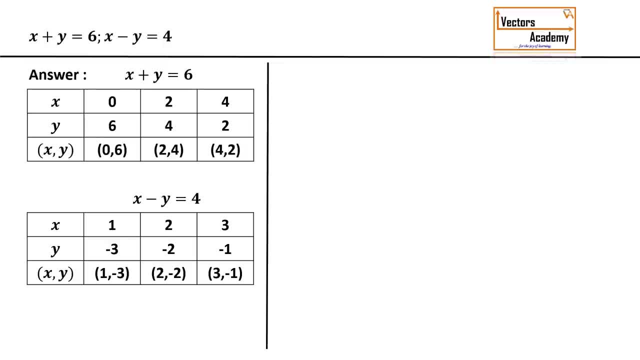 which are to be plotted on the graph Once we have made the table for both the lines. we'll take the second value of x, that is, x equal to 2, and substitute in the equation. Again, I'll get three points which are to be plotted on the graph Once we have made the table for both the lines. we'll take the second value of x, that is, x equal to 2, and substitute in the equation- Again, I'll get three points which are to be plotted on the graph Once we have made the table for both the lines. we'll take the second value of x, that is x equal to 2, and substitute in the equation- Again I'll get. three points which are to be plotted on the graph Once we have made the table for both the lines. we'll take the second value of x, that is, x equal to 2, and substitute in the equation. Again, I'll get three points which are to be plotted on the graph Once we have made the table for both the lines. 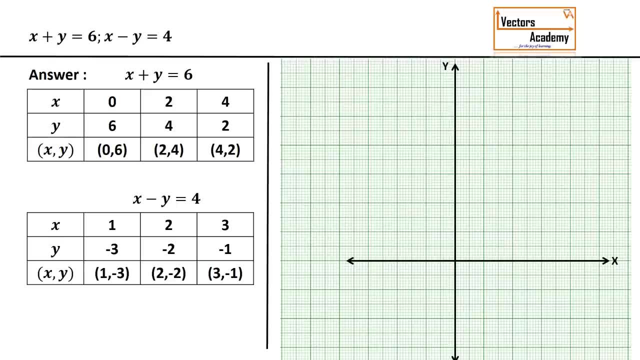 we'll take the second value of x, that is, x equal to 2, and substitute in the equation Again, I'll get these lines. Now we have the x-axis and the y-axis. The scale on both the axis is usually taken as one centimeter, as one unit. Now for the first line, the first. 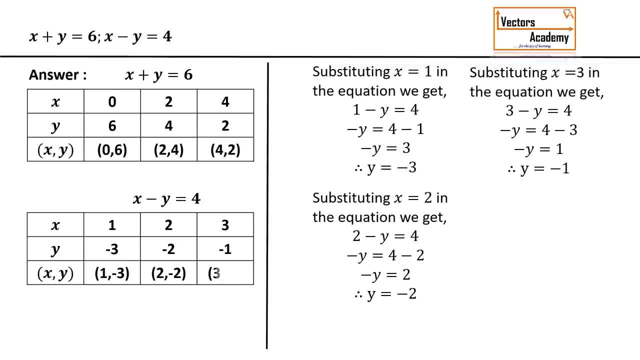 the equation and I'll get the value of y as minus 1.. Again, I'll get three points which are to be plotted on the graph Once we have made the table for both the lines. now we can take our graph paper and plot these lines. Now we have the 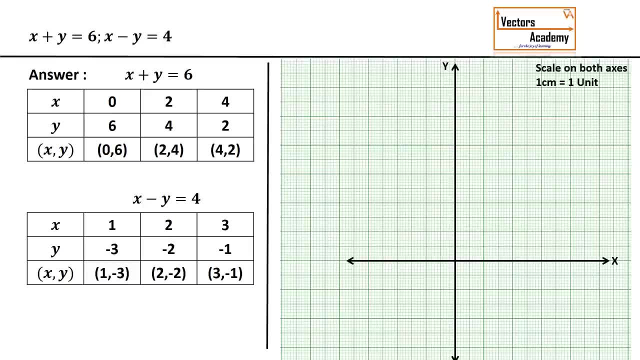 x-axis and the y-axis. The scale on both the axis is usually taken as 1 centimeter, as 1 unit. Now for the first line. The first point is 0, 6, which lies on the y-axis. The second point is 2, 4, because we have x coordinate 2, y coordinate 4.. The third: 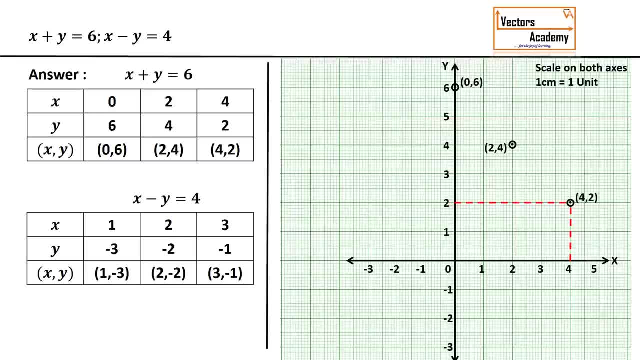 point is 4, 2, because we have x coordinate 4, y coordinate 2.. So after plotting these three points, I will join them and I will get the required line, that is, x plus y, equal to 6. now we'll put the second line on the same graph: 1 minus 3. 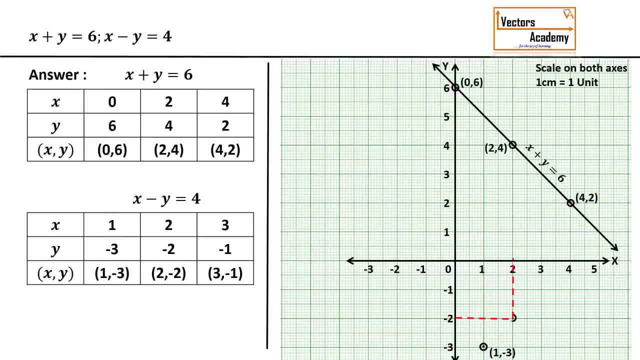 x coordinate 1, y coordinate minus 3, again, 2 minus 2 and 3 minus 1- again. I will join them. I'll get the second line now. once you have drawn both the lines, you have to find out where both of these lines intersect. so these lines. 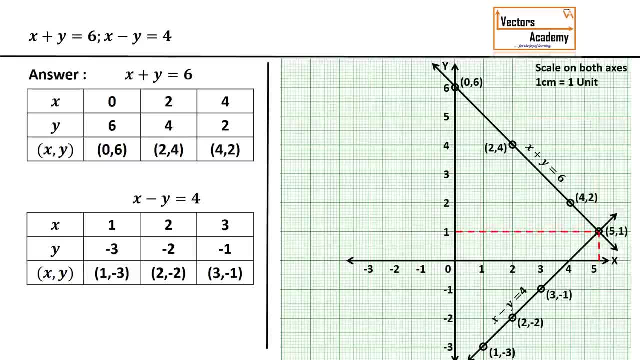 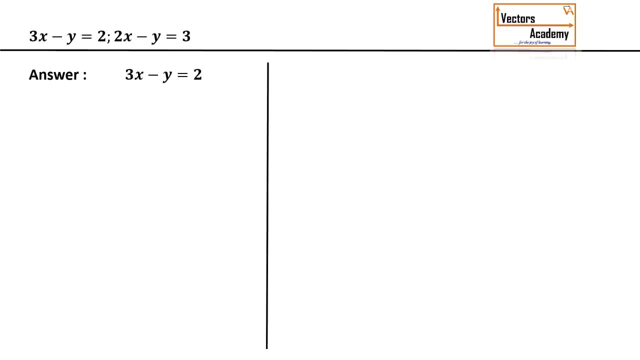 intersect at a point whose x coordinate is Phi and y coordinate is one, right. so that's the answer for this question: X is Phi and Y is 1. so this is how we solve equations using graph. let's have another example of this type. we have have two equations: 3x minus y equal to 2, and 2x minus y equal to 3. now again, we'll take the first. 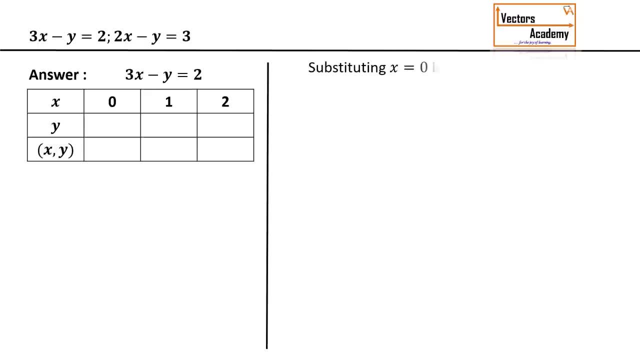 line. we'll make the table. we'll assume the values of x and substitute them one by one. so if i substitute x equal to 0, i'll get y is equal to minus 2. if i take x equal to 1, i'll get y is equal. 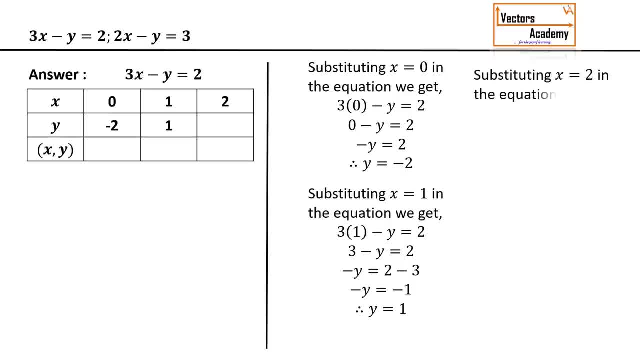 to minus 1. if i take x equal to 2, i'll get the value of y as 4. so once i get these points, i can plot these points and make the graph of the first line exactly in the same way. the second linear equation is given. i'll assume the values of x. i'll substitute them in the equation of line. 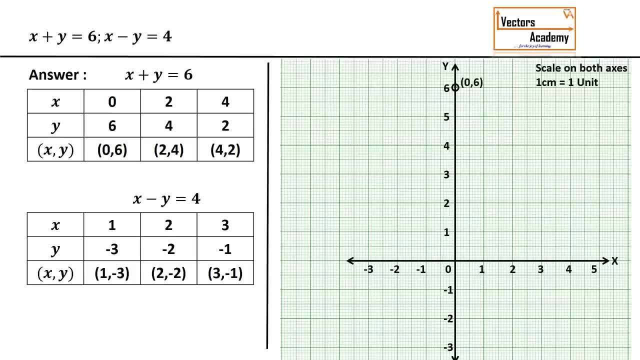 point is 0,6, which lies on the y-axis. The second point is 2,4, x coordinate 2, y coordinate 4.. The third point: 4,2, x coordinate 4, y coordinate 2.. So, after plotting these three points, I will join them and I'll get the required line that. 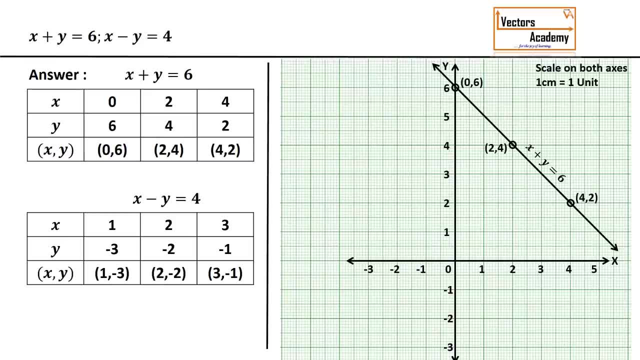 is x plus y equal to 6.. Now we'll plot the second line on the same graph: One minus three, x coordinate 1,. y coordinate minus three. Again, two minus two and three minus one. Again, I will join them. I will get the second line Now, once you have. 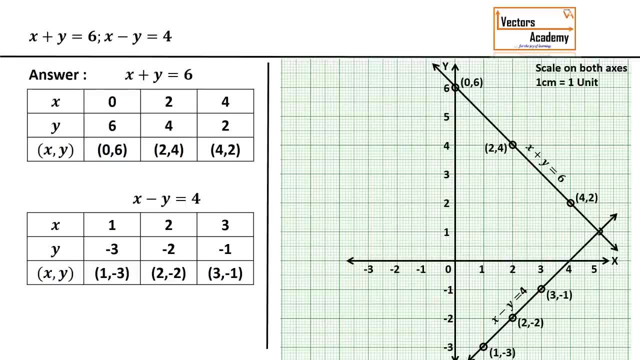 drawn both the lines, you have to find out to where both of these lines intersect. So thisision has important, important to find outون. So these lines intersect at a point whose x coordinate is 5 and y coordinate is 1, right. 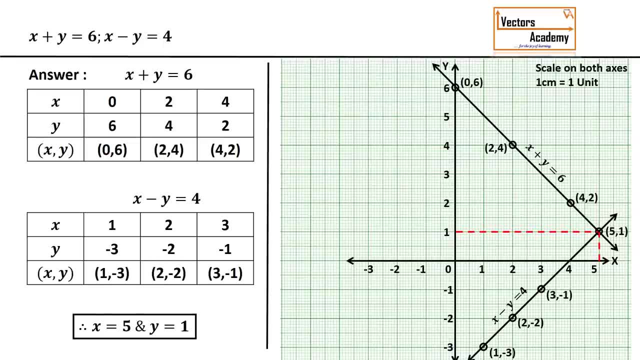 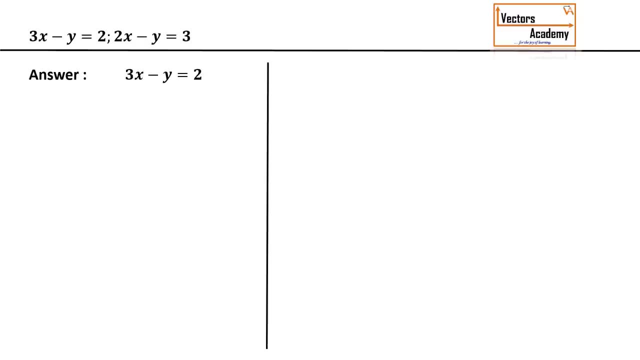 So that's the answer for this question: X is 5 and y is 1.. So this is how we solve equations using graph. Let's have another example of this type. We have two equations: 3x minus y, equal to 2, and 2x minus y, equal to 3.. 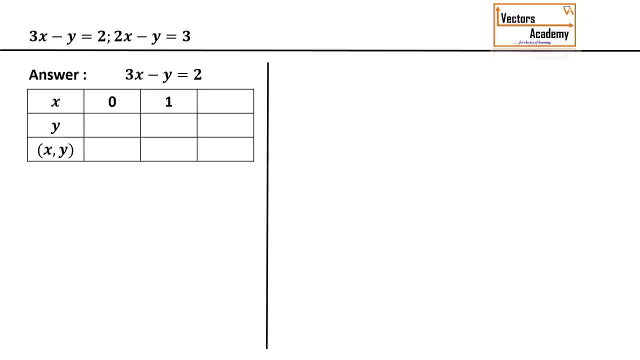 Now again, we'll take the first line, we'll make the table, we'll assume the values of x and substitute them one by one. So if I substitute x equal to 0, I'll get y is equal to minus 2.. If I take x equal to 1, I'll get y is equal to minus 1.. 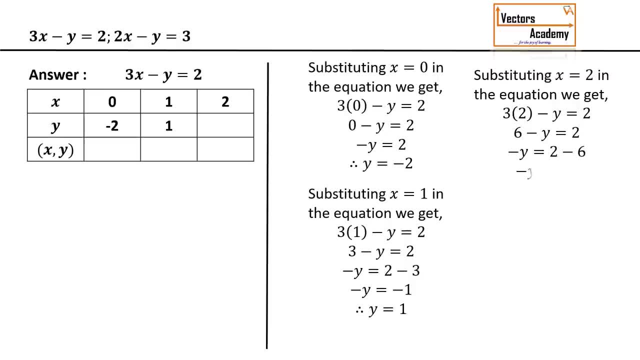 If I take x equal to 2, I'll get y is equal to minus 1.. I'll get the value of y as 4.. So once I get these points, I can plot these points and make the graph of the first line. 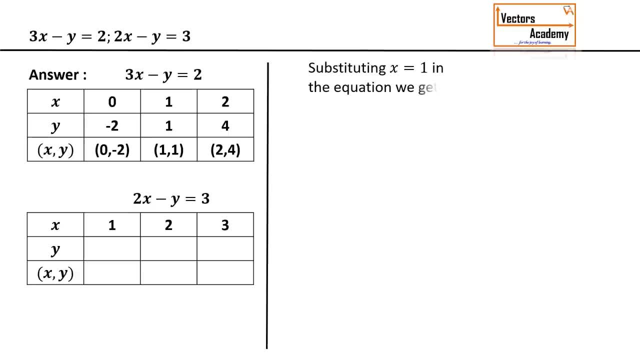 Exactly in the same way. the second linear equation is given. I'll assume the values of x, I'll substitute them in the equation of line and I'll find out corresponding values of y as well. Now, once we have got all the three points, we can again take the graph paper. we can